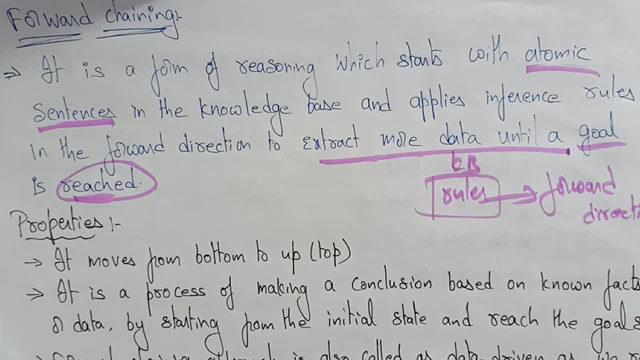 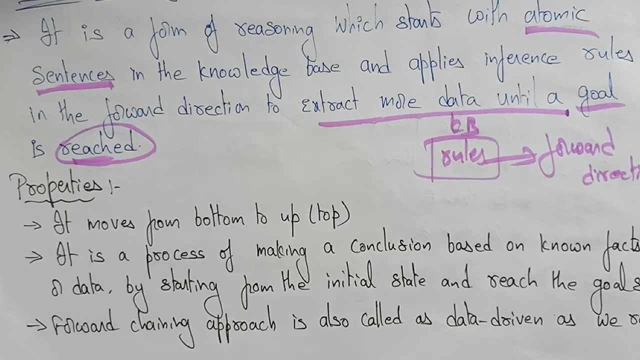 that main aim here is extract more data until a goal is reached. There is a concept of the forward chaining. Now let's see the properties of this forward chaining. A forward chaining moves from bottom to top. The thing here is it moves from bottom to top. First takes the first rule. 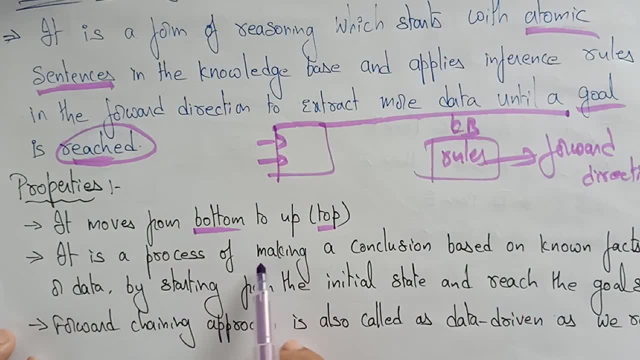 second rule: like that it moves from bottom to top. It is a process of making a conclusion based on known facts or data. So the forward chaining is a process of making a conclusions. what type of conclusions means it has to reach the goal So that conclusions are based on known. 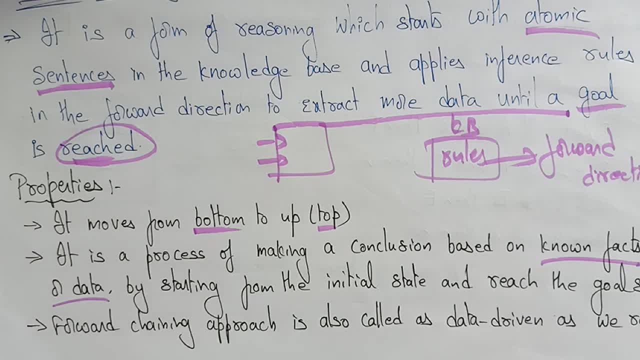 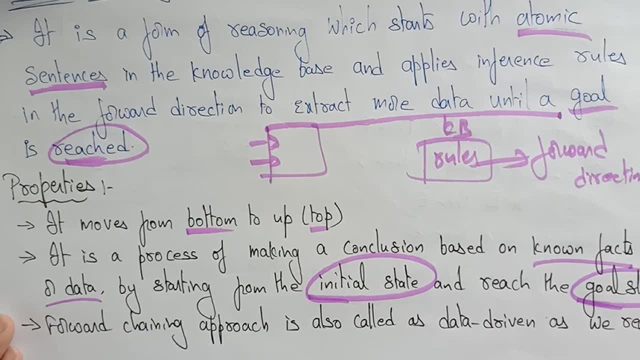 facts or data. So by starting from the initial state and reaches the goal state. So always it starts with the initial state and finally it reaches to the goal state. It is a forward direction, taking the initial steps and reaches the final steps, The forward chaining approach. 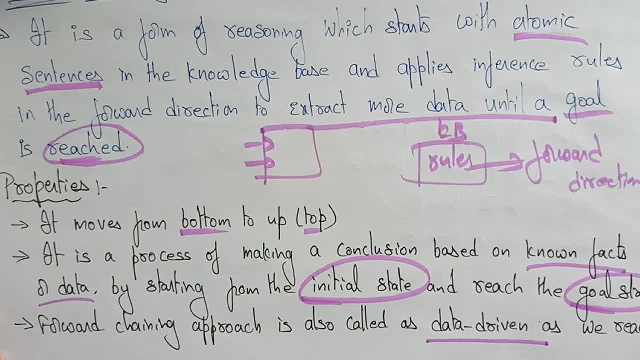 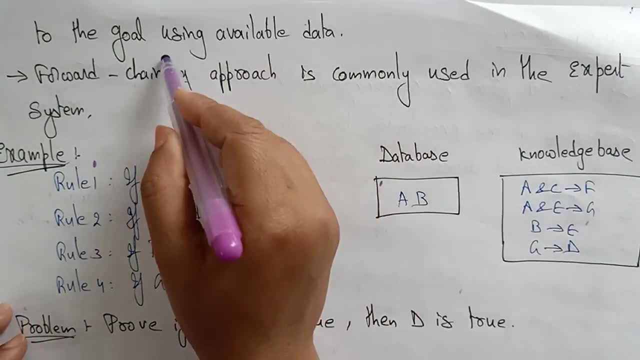 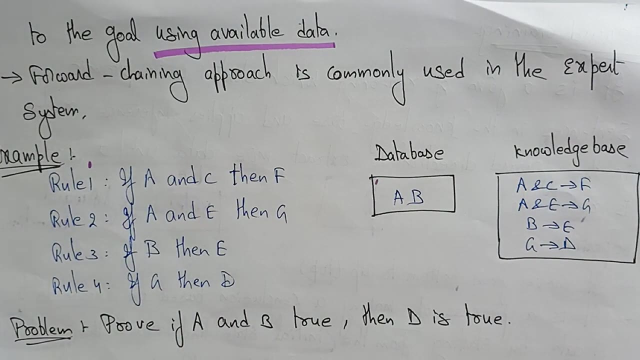 is also known as the data driven. Why we call it as a data driven? because as we reach to the goal using the available data, So with the help of the available data, we are reaching the goal. So that's why we call it as the forward chaining is also called as a data driven. 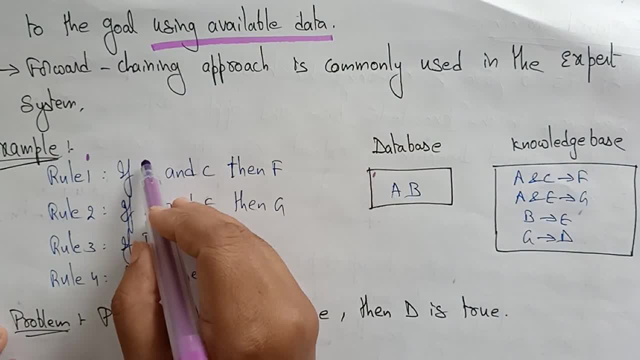 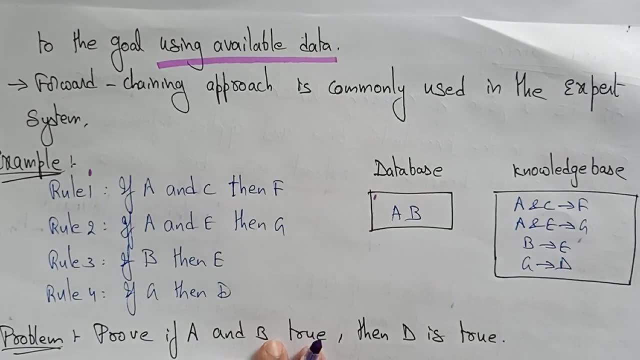 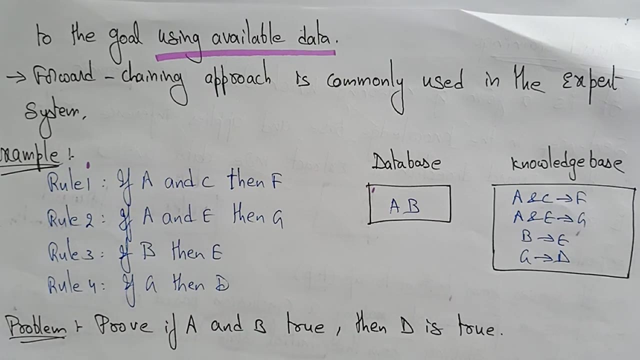 The forward chaining approach is commonly used in the expert systems. Okay, remember that it will be used in the expert systems. Let's see some of the example of forward chaining, how the forward chaining will be taking place. So, with the help of the content, we are reaching the goal state. 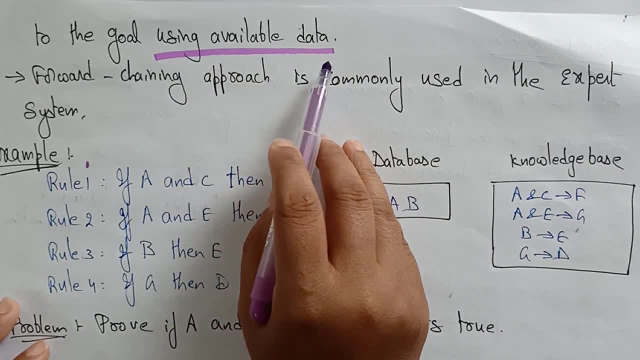 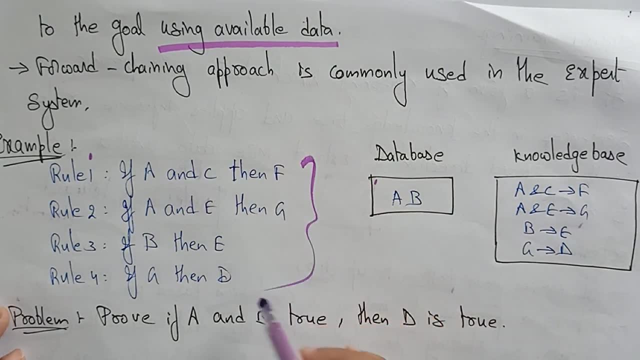 Again, that is the data that is available. on the available data and with the help of the set of the rules, we are going to reach the goal. Let's see here. So here some of the rules are there which are present in the knowledge base. Okay, so these rules are placed on the knowledge base If A and C 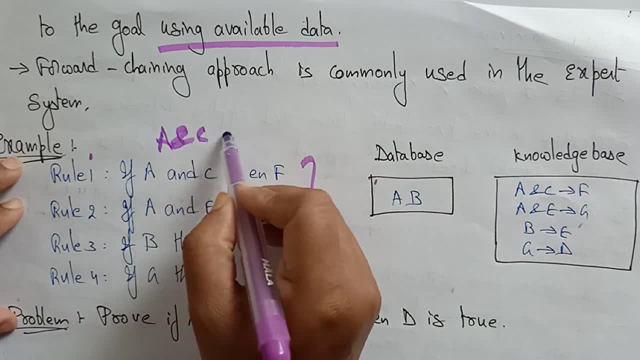 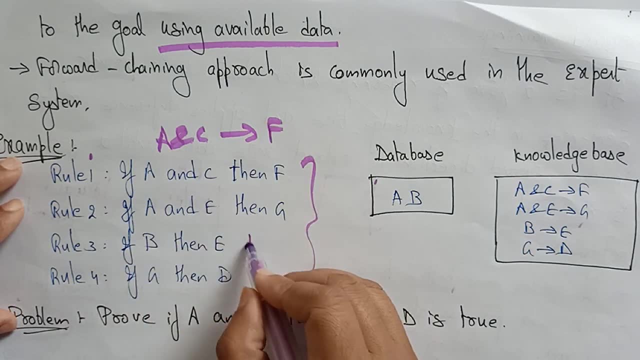 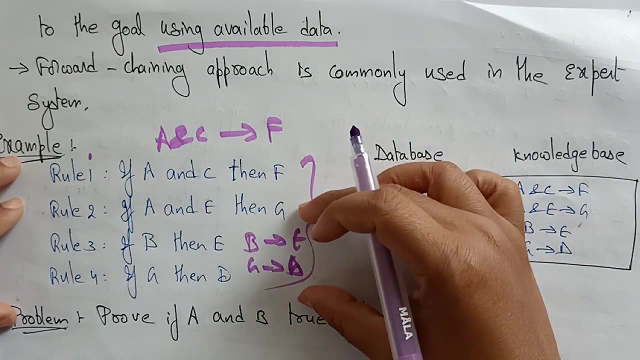 then F. Okay, that means A and C, then F. If A and D, then G. If B, then E means that is B implies E, So G implies D. So these are the some rules. they are given. So, based on the rules and the data, 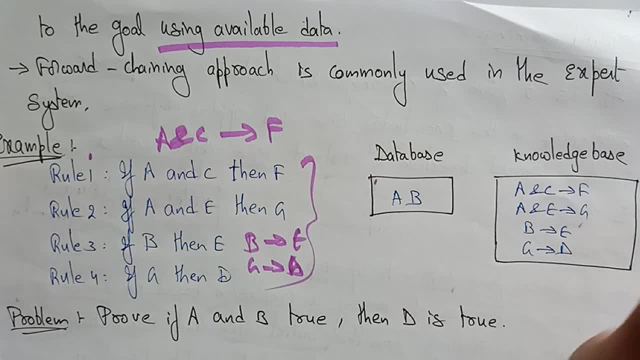 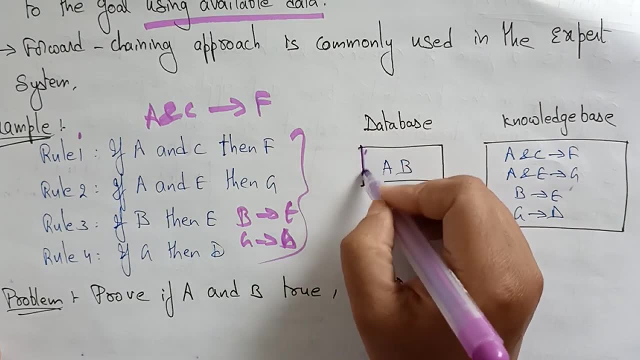 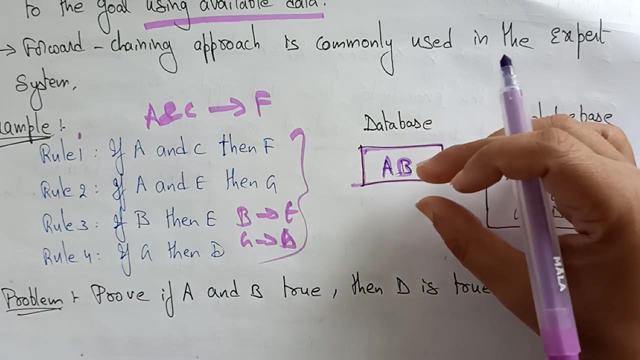 that is available. we have to reach the goal. So prove: if A and B true, then D is true. So that means AB is already it is there in the database, means it is already fixed. Some data, that is already satisfied, that data is present on the database. So finally, the D is also has to reach. 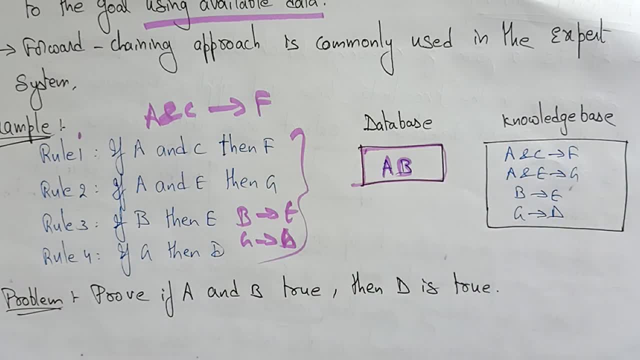 the database. Whenever the data is present on the database, it is already fixed. So finally, the D has reached the database. then our condition is satisfied, means we reached the goal. So here the problem is we have to prove: if A and B is true, then D is also true. So A and B I am taking it. 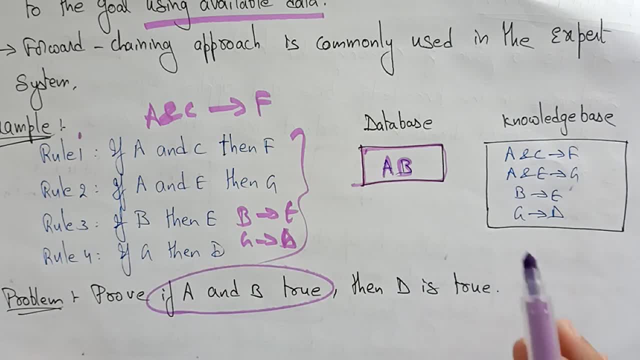 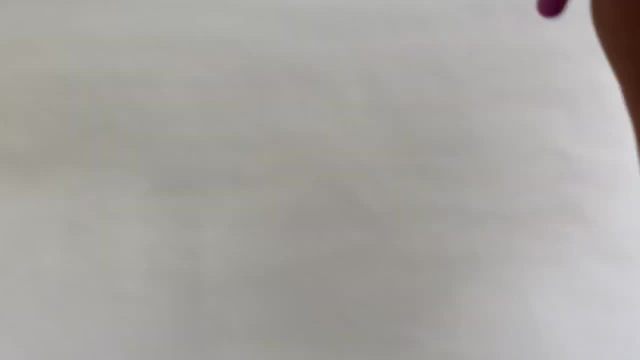 as a true and I have to execute D in the database. So that is a concept. Now let's start the problem: How I am going to execute. Let's see So by using the forward chaining. So here what? 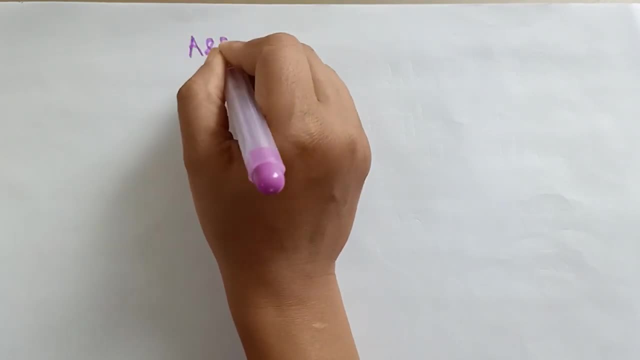 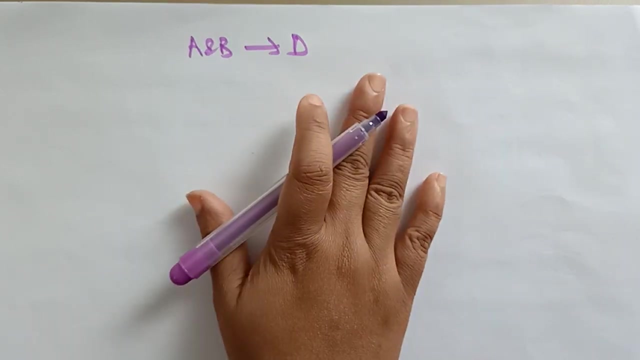 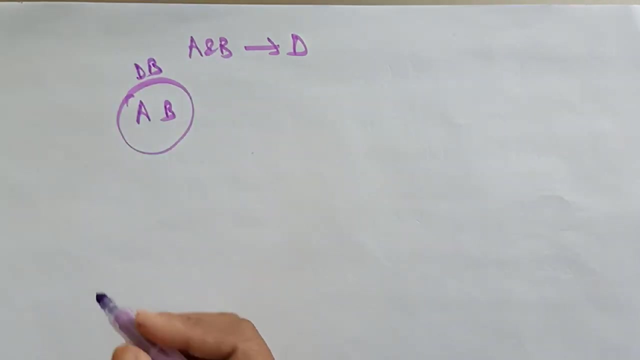 they are saying: I have to prove if A and B is present, then D is also present. So here what they are saying I have to prove: if A and B is present, then D is also satisfied. I have to prove this. So initially, what it is having Initially AB is present in the database. So in the knowledge. 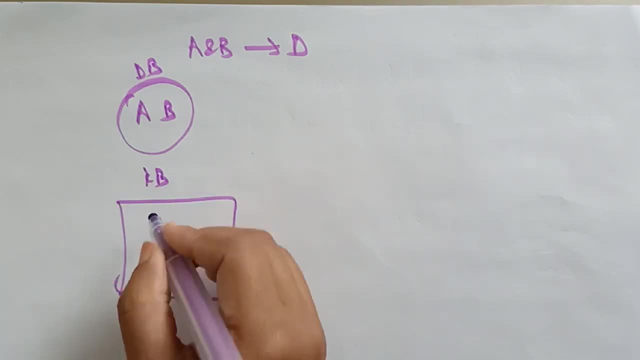 base, we are having the set of rules. What are the set of rules it is having? A and C implies E, A and E implies G, and B implies E And G implies D. So these are the set of rules that are present in the knowledge base. Now I need 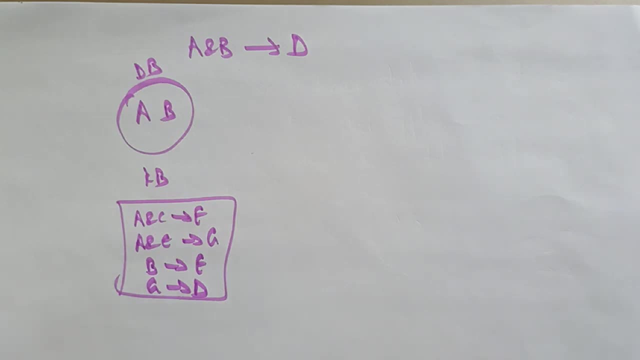 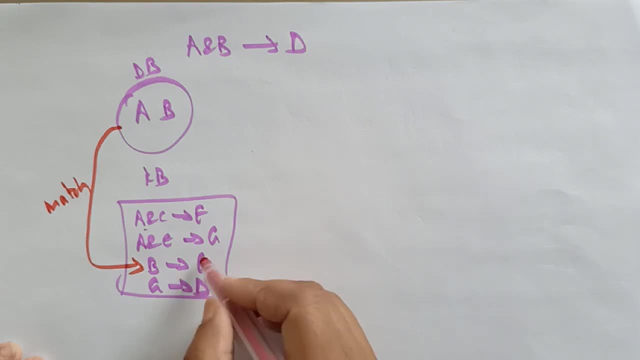 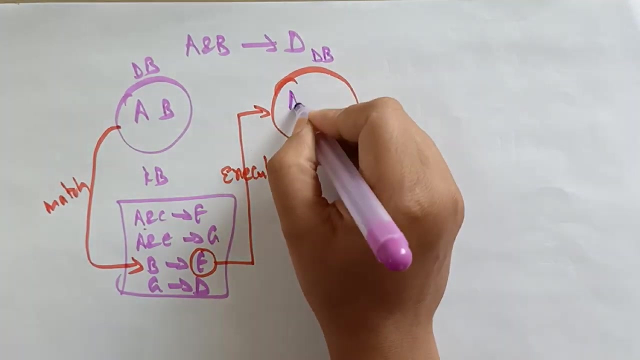 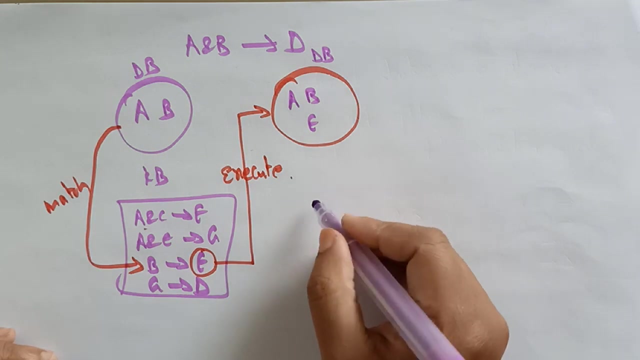 B implies E, B implies E. That means I have to place this E on database, That is, execute, Execute E in database. Now the database contains what? the items the database contains: A, B, E. Now check. So this is my knowledge base. Okay, So my knowledge base is this. So A and C implies 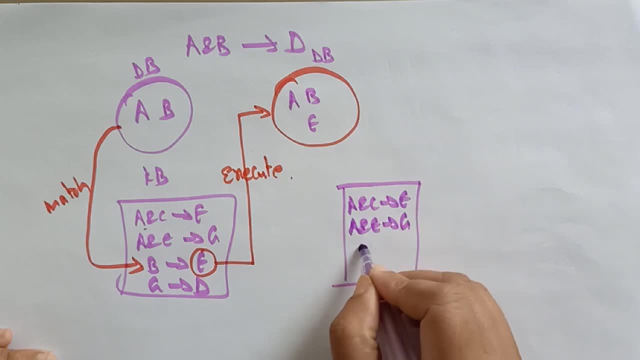 E. A and E implies G, B implies E and G implies D. Now check A- B combination. is there No B combination already? I visited A and E combination is there Means A and E combination is there. So 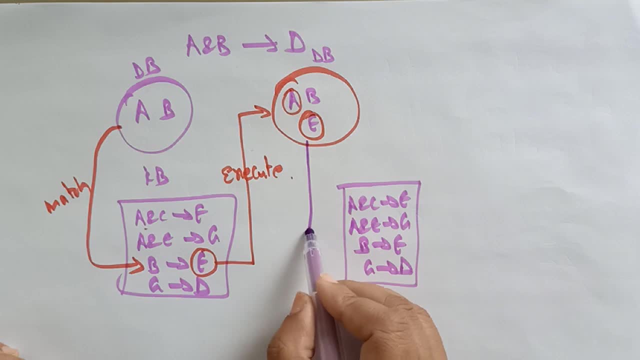 I have to. with the help of elements in database, I am going to execute A and E. So what is our A and E implies G, So this is matching To the knowledge base. So, whatever the element that is A and E implies that G has to be execute. 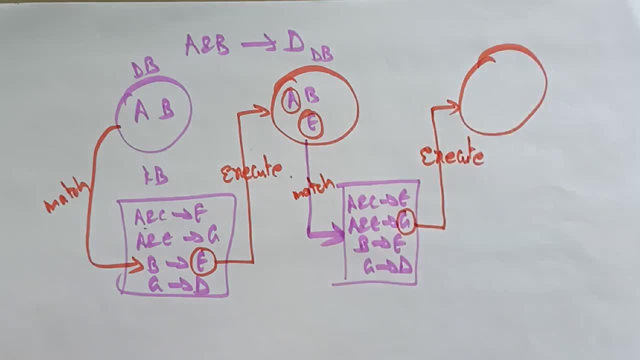 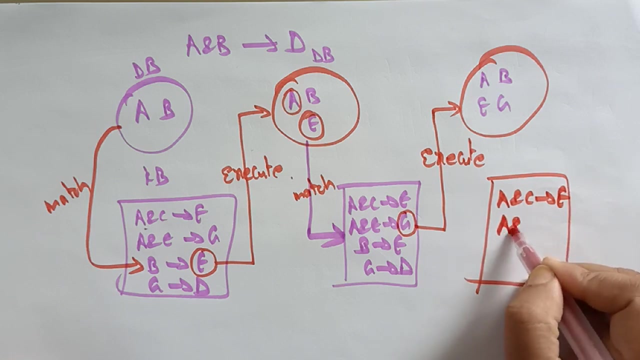 in database. So now the database contains A, B, E and G. Okay, So now again match here: A and C implies E, A and E implies G, B implies E and G. So now check: Single A is not there. A and B is not there. Okay, Single E is also not there, It's. 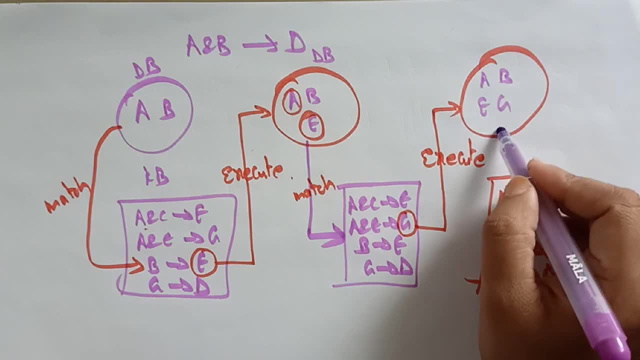 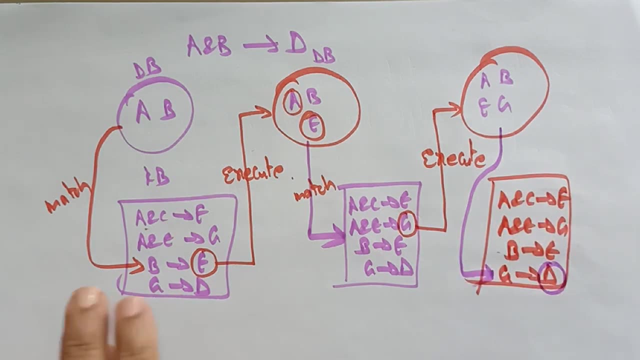 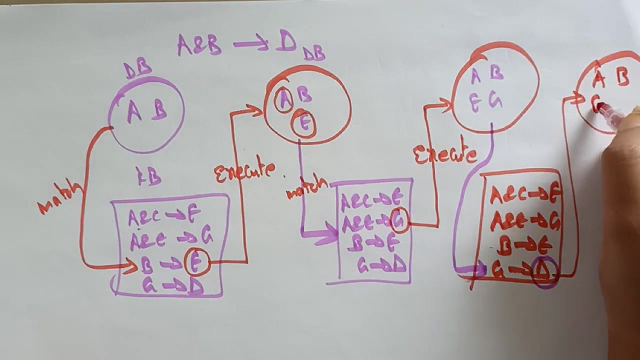 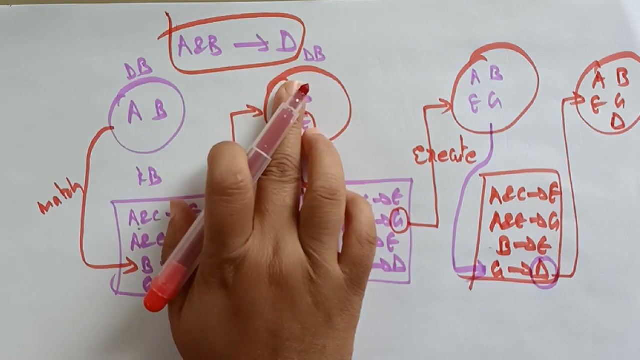 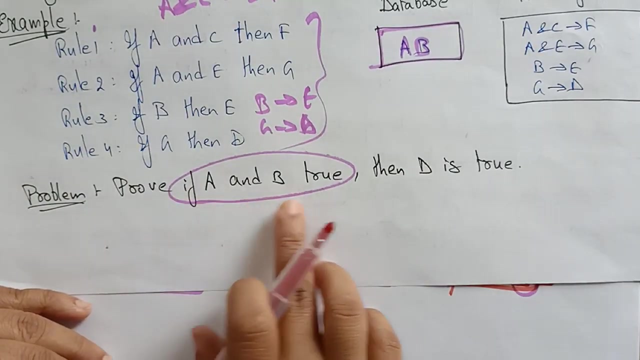 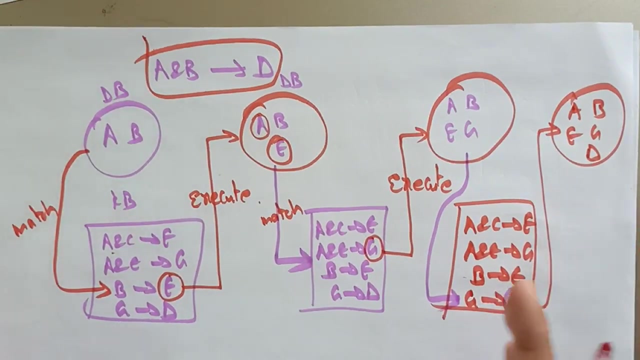 not matching. Single G is there Means G is matching with this item in the knowledge base. So then execute this D in database. So now the database contains A, B, E, G and D. So did we reach with the goal? Yes, we reached with the goal. A and B implies D Means whenever the A and B are executed, then D is also executed. So we proved that If A and B is true, then D is also true. So whenever it is executed in the database means it is true. So this is a way of doing the forward chaining. So in the next video I will take one more example to clarify your doubt. Thank you,